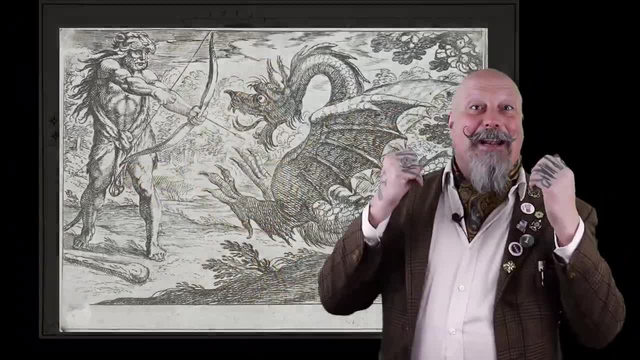 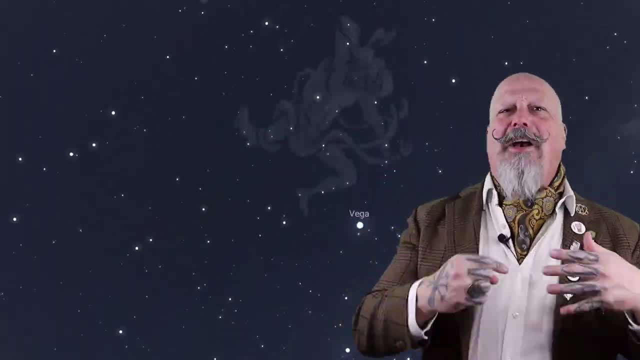 Hercules performed 12 labors, the penultimate of which involved defeating the dragon Ladon so he could steal the golden apples of the Hesperides. If you look towards the north, we see Hercules triumphant standing upon the head of Draco. Draco is Latin for dragon and is 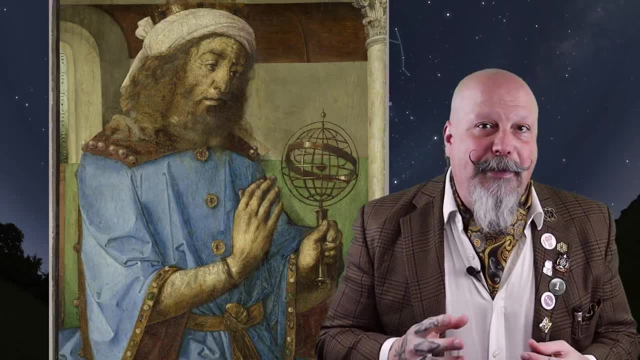 also one of the largest constellations in the sky. When Ptolemy named the original 48 constellations back in the 2nd century, Draco was amongst them and is still one of the 88 constellations today. 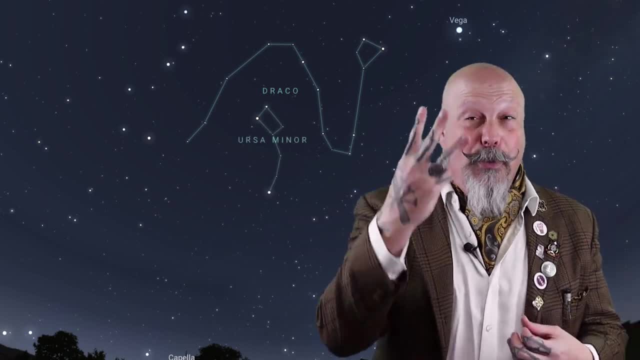 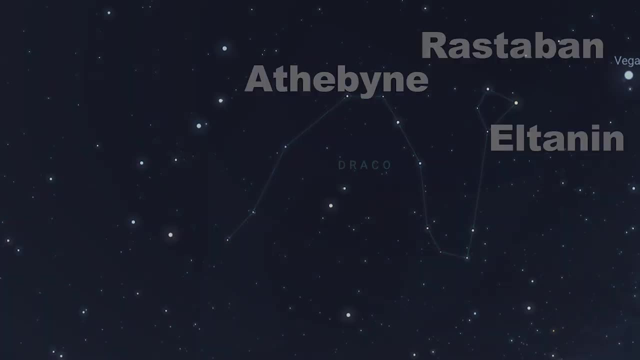 Draco slithers across the sky, hugging Ursa Minor, and contains three very bright stars: El Tannin, Athabine and Rastaban. See if you can spot them. junior scientists, It's your last chance to dance this summer with our friend Venus. Venus has been lighting our western skies since spring, but will start setting before sunset. later in the month, On July 9th, Venus will be at its brightest setting just after sunset. Look to the west While we say goodbye to Venus, the gas giants Saturn and Jupiter. 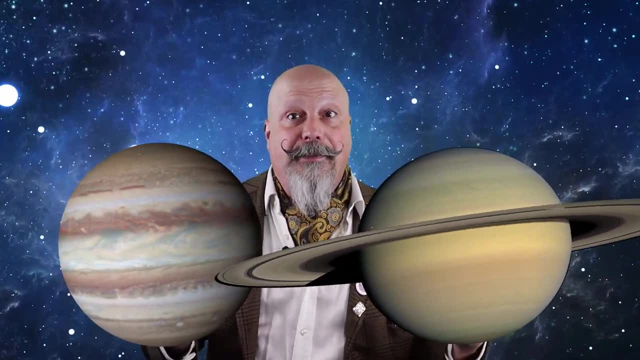 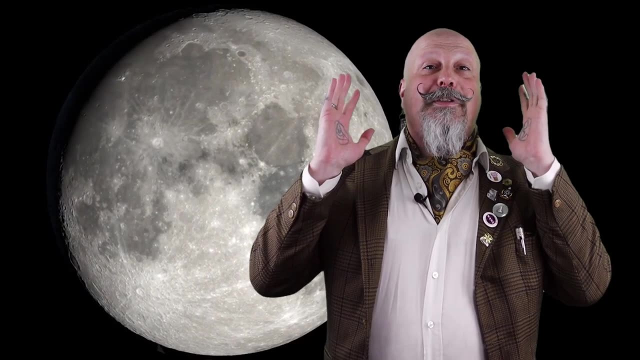 increase in visibility in the early mornings in the south and southeast. Bright and high in the sky. they'll be visible in the hours just before dawn. The full moon this month is on July 3rd and it's actually the first of four supermoons this year. 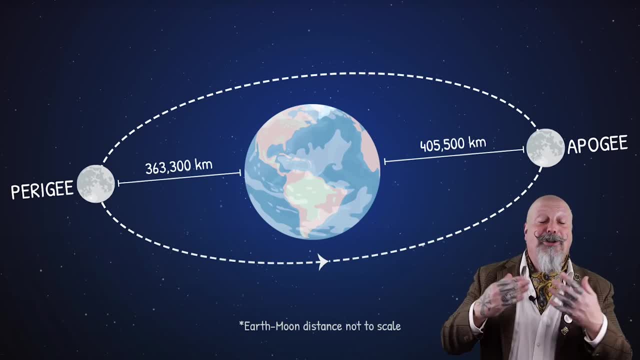 What's a supermoon? The moon's orbit around the Earth is not a perfect circle. it's actually an ellipse. This means there's a point in the orbit where the moon is not a perfect circle. This means there's a point in the orbit where the moon is furthest from the Earth, called apogee. and a point where it's closest to the Earth, called perigee. July 3rd is not only a full moon, but it's also perigee, where the moon is actually 40,000 kilometers closer to the Earth. As a result, 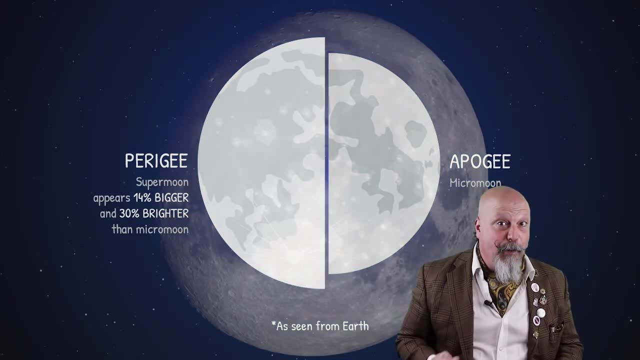 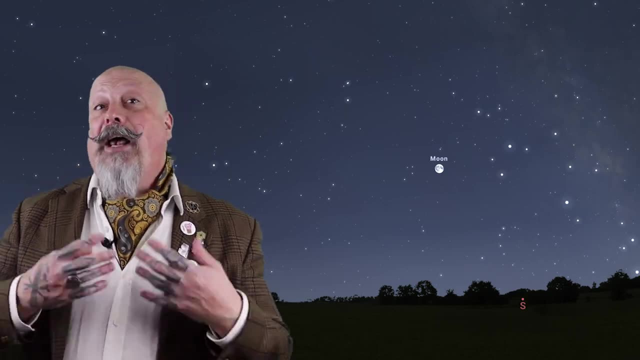 it appears larger in the sky. As I mentioned before, this is the first of four supermoons this summer, with two in August and one at the end of September. to round out, our summer Settlers commonly refer to the July full moon as the buck moon or the thunder moon. 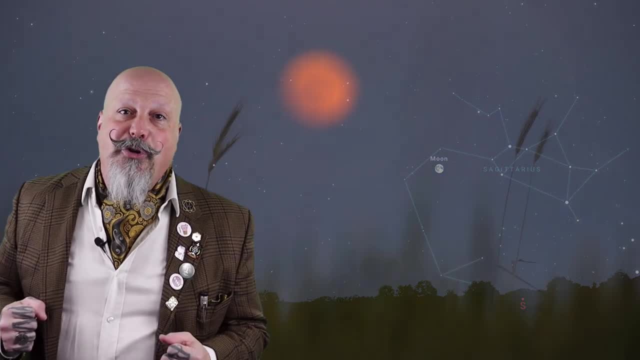 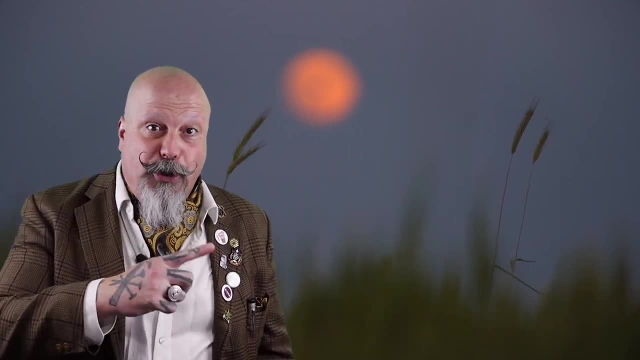 and is found inner near the constellation Sagittarius. This moon is referred to by the Anishinaabe of the Great Lakes region as the halfway summer moon. This is because the days have already started to shorten after the summer solstice back in June. The Cree of Central Canada. 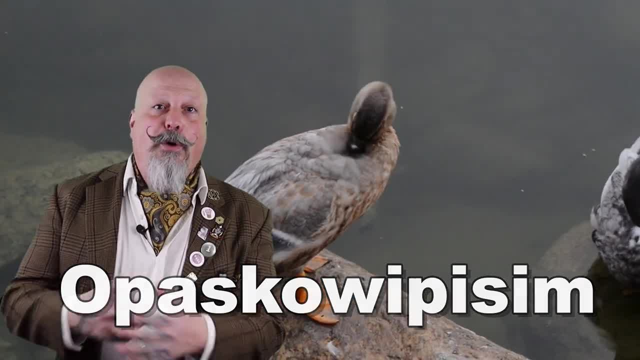 call the July full moon Opaskawi Pism, the feather-molting moon, in reference to the water fowl, And the Mi'kmaq of the East Coast also refer to this behavior, calling it Beskewi Goose. 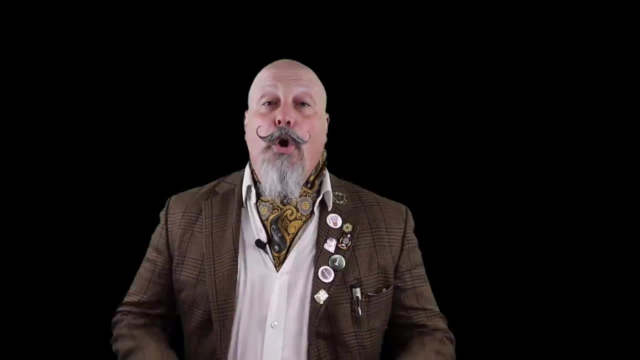 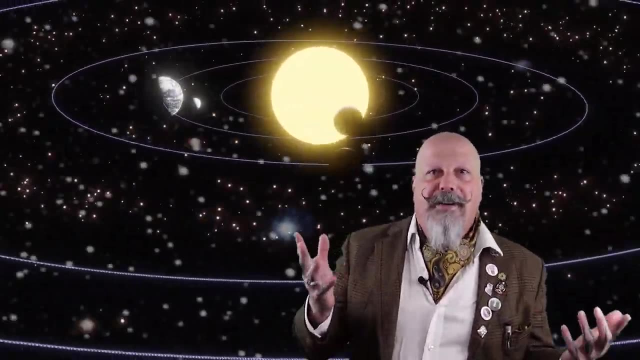 the bird-shedding feathers moon. We'll wrap up this month with a cool summertime phenomenon you can try and spot. As you may know, our home, the Earth, spirals around our sun within a moving galaxy called the Milky Way.